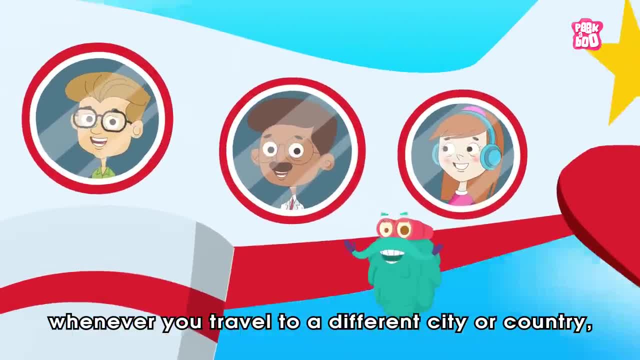 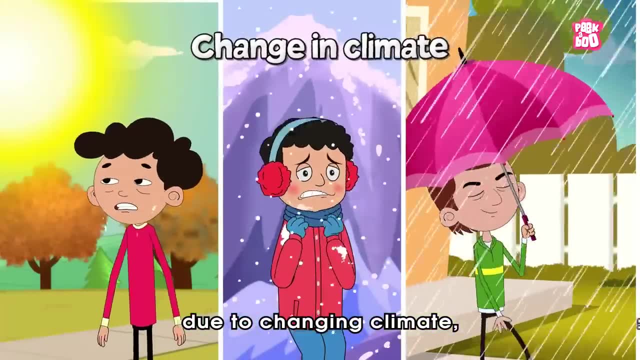 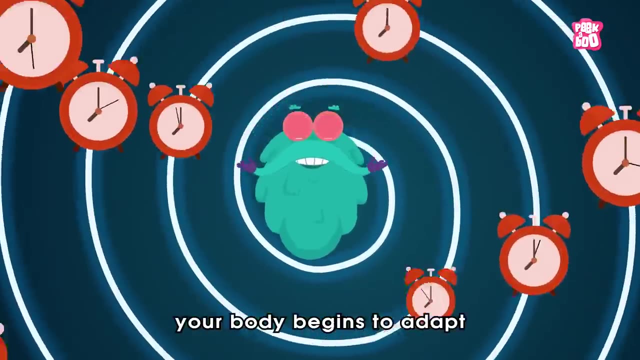 As you must have seen, whenever you travel to a different city or country, you find it extremely difficult to adjust to it for a while due to changing climate, food or water. But as time progresses, your body begins to adapt to the new environment. that helps you. 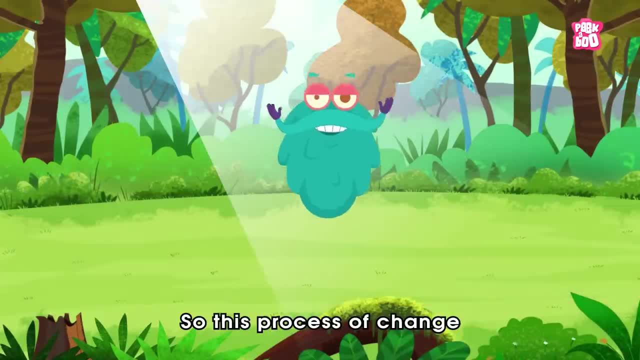 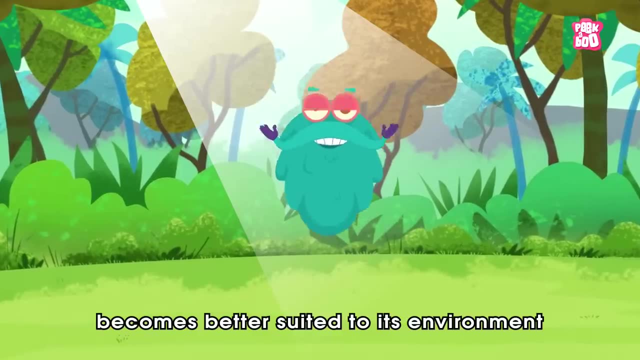 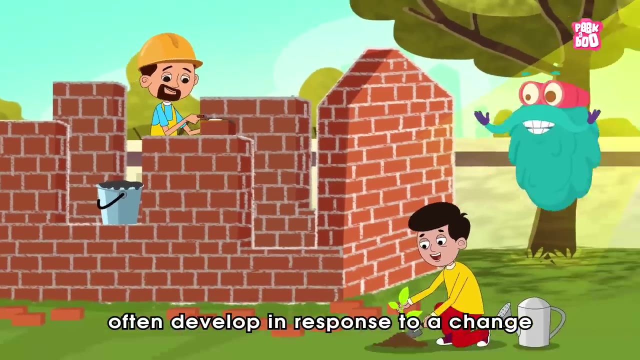 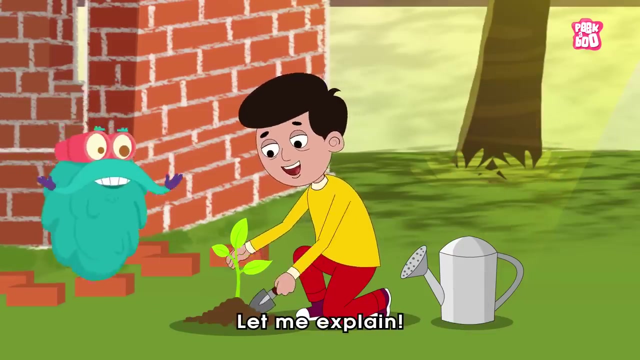 to feel better and settle down. So this process of change, by which an organism or species becomes better suited to its environment, is called adaptation. In other words, adaptations often develop in response to a change in the organism's habitat, and the same is the case with the plants. 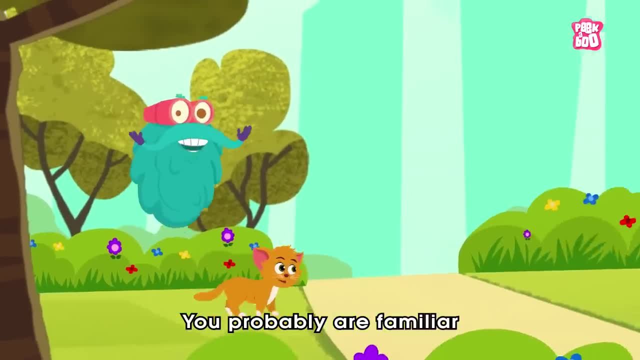 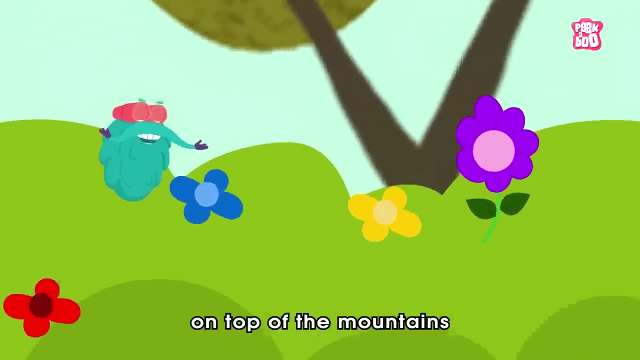 Let me explain. You probably are familiar with the plants in your environment. Yes, you are familiar with the plants in your environment. Yes, you are familiar with the plants in your environment. They are everywhere: over the land, on top of the mountains and under water. 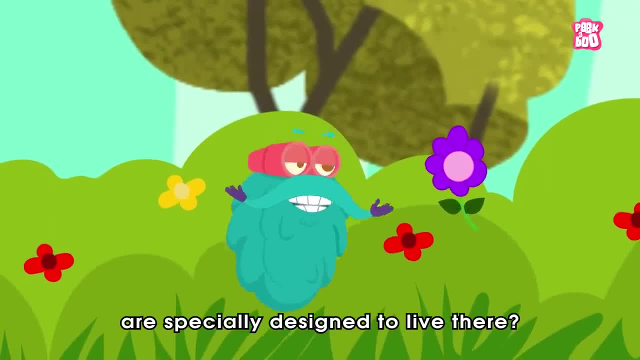 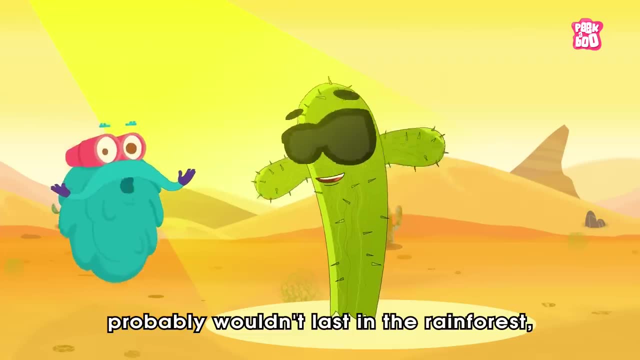 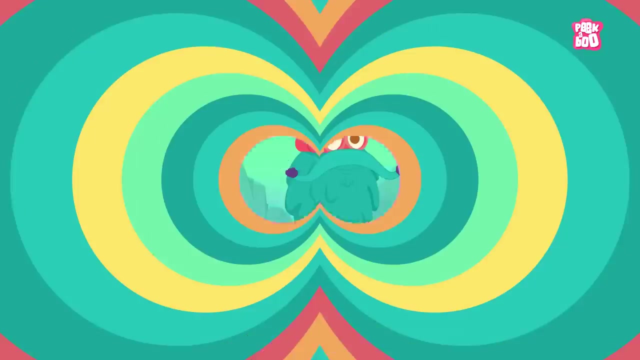 But did you know that those plants are specially designed to live there? Yes, a tree that lives in the desert probably wouldn't last in the rain forest, and a tall tree can't survive in grasslands. The reason plants are able to survive in their environment is because they are able to survive. 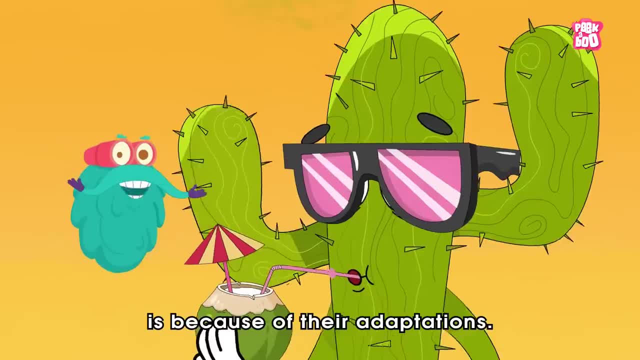 in the rain forest. The reason plants are able to survive in their environment is because they are able to survive in the rain forest, and a tall tree can't survive in the rain forest. They are able to survive in the rain forest because of its adaptations. 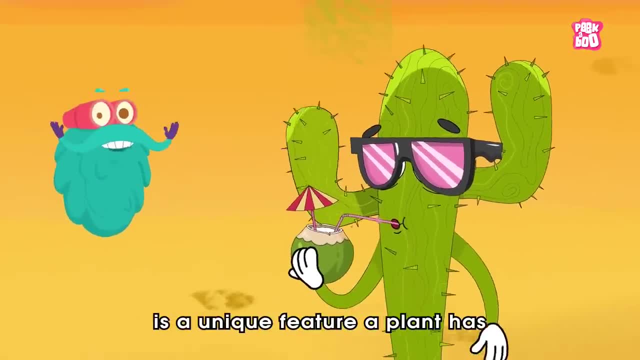 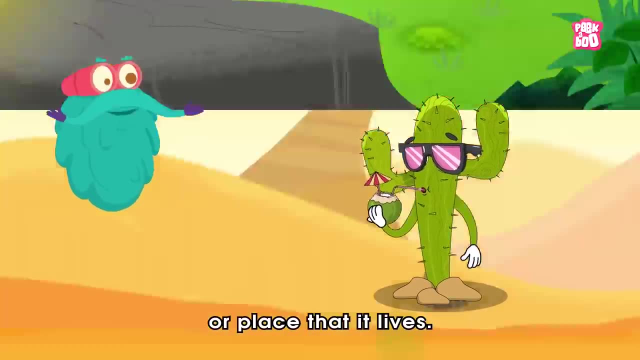 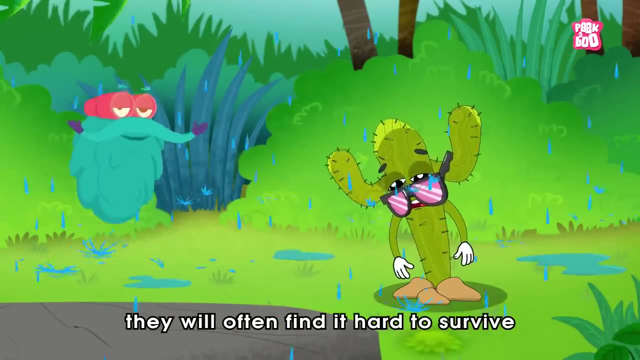 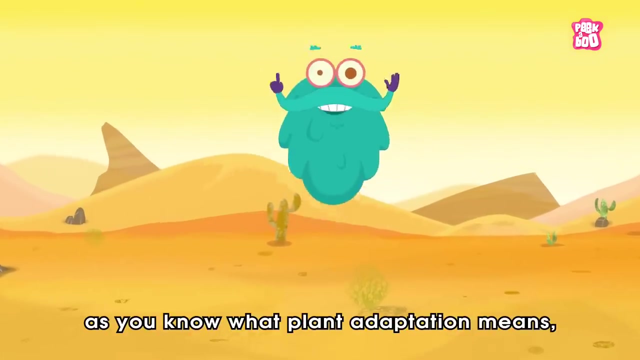 A plant. adaptation is a unique feature a plant has that allows it to live and grow in its habitat or place that it lives, And once you move these trees from their natural habitat, they will often find it hard to survive and eventually die. So now, as you know what plant adaptation means, 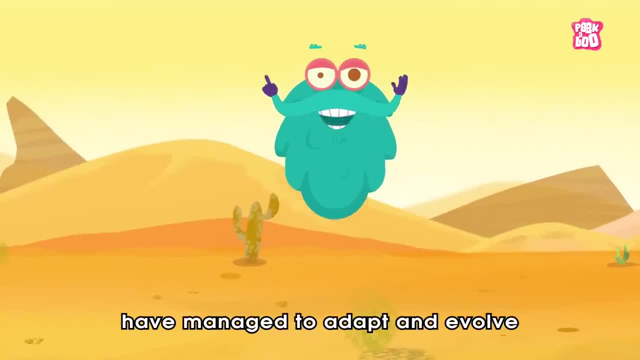 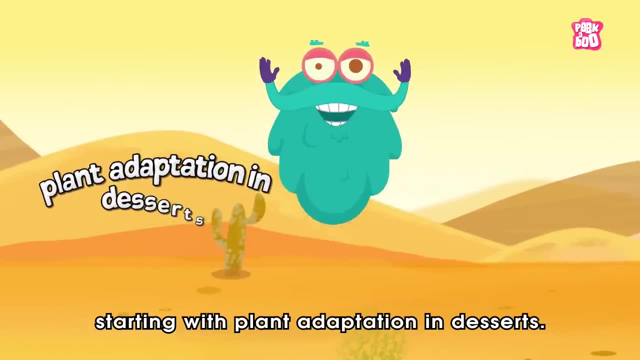 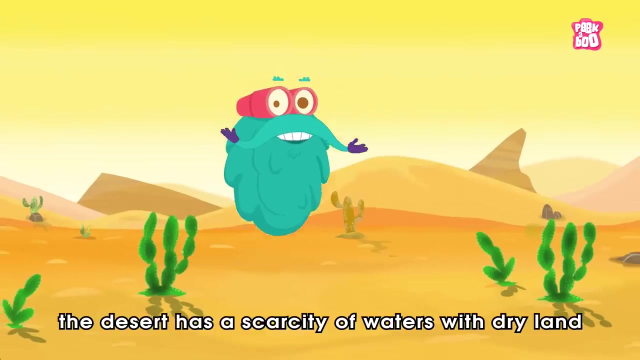 Now let us briefly look at this. So now let us briefly look at this. Look at how these trees have managed to adapt and evolve according to their habitats, starting with plant adaptation in deserts. As we know, the desert has scarcity of water, with dry land. 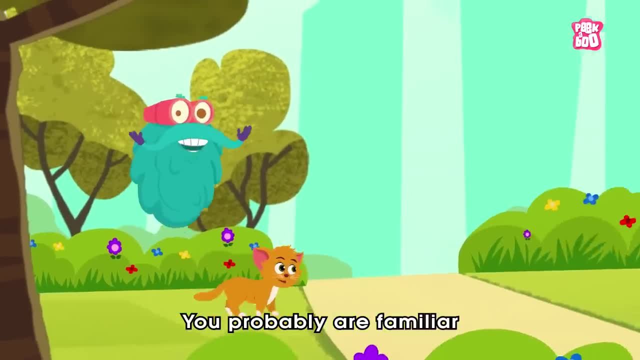 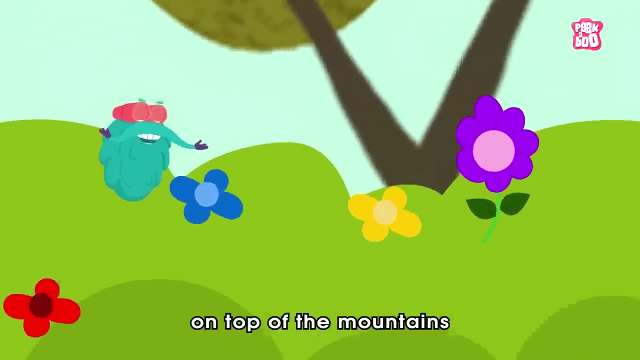 Let me explain. You probably are familiar with the plants in your environment. You may be familiar with the plants in your environment. You may be familiar with the plants in your environment. They are everywhere: over the land, on top of the mountains and under water. 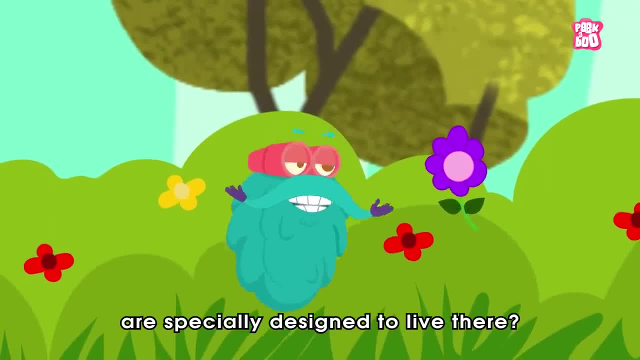 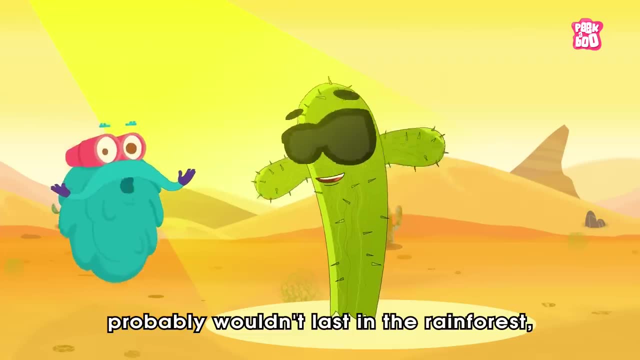 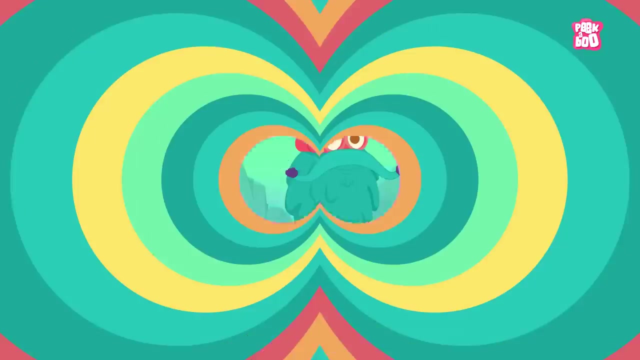 But did you know that those plants are specially designed to live there? Yes, a tree that lives in the desert probably wouldn't last in the rain forest, and a tall tree can't survive in grasslands. The reason plants are able to survive in their environment is because they are able to survive. 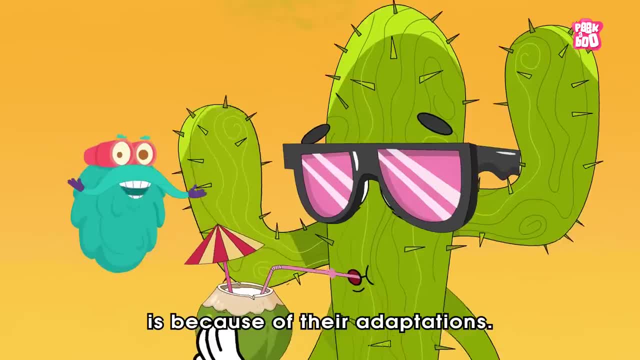 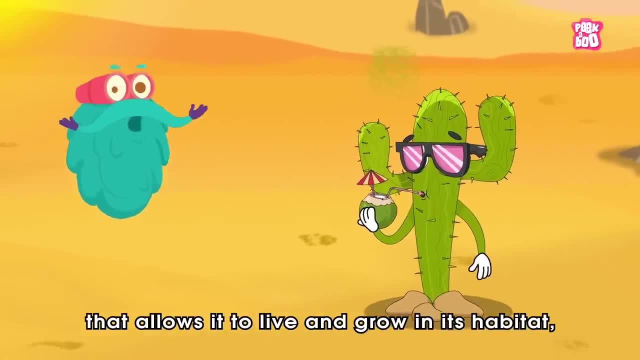 in the rain forest. The reason plants are able to survive in the rain forest is because they are able to survive in the rain forest. The reason plants are able to survive in the rain forest is because of its adaptations. A plant adaptation is a unique feature a plant has that allows it to live and grow in its 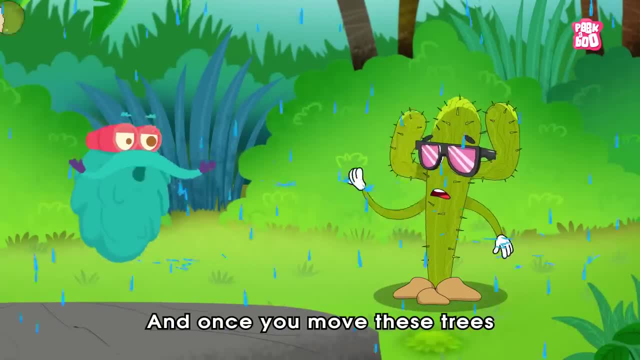 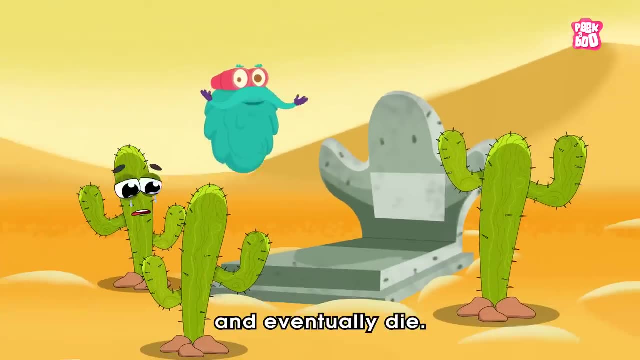 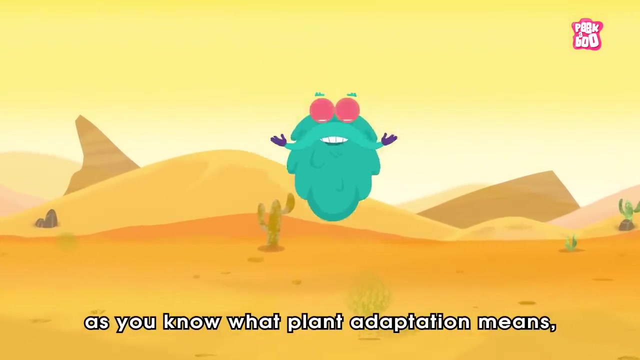 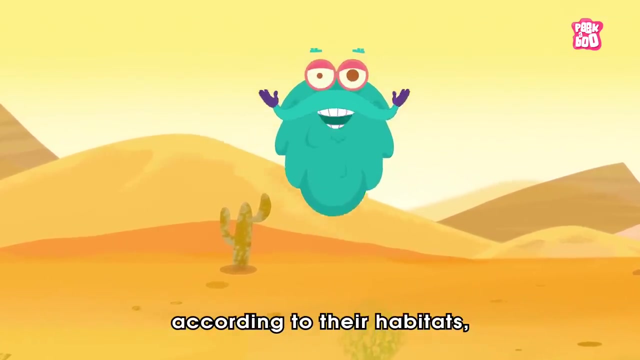 habitat or place that it lives. And once you move these trees from their natural habitat, they will often find it hard to survive and eventually die. So now, as you know what plant adaptation means, let us briefly look at the plant adaptation looked at how these trees have managed to adapt and evolve according to their habitats. 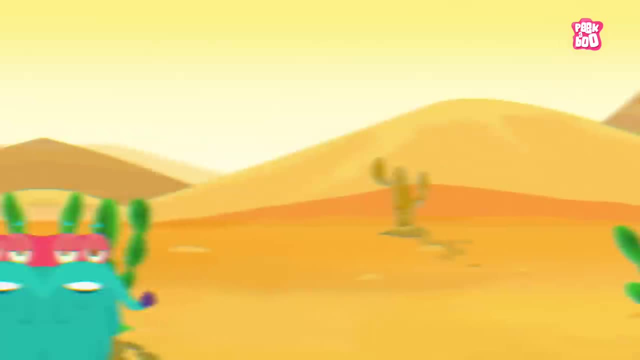 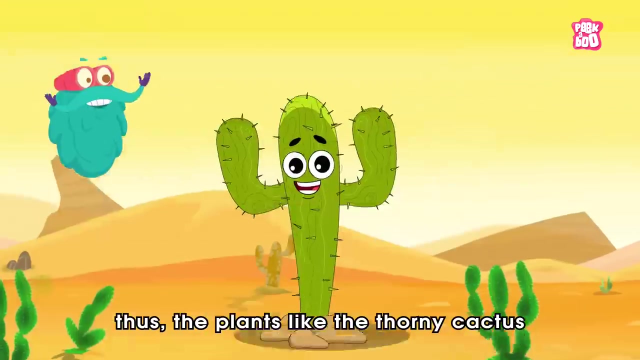 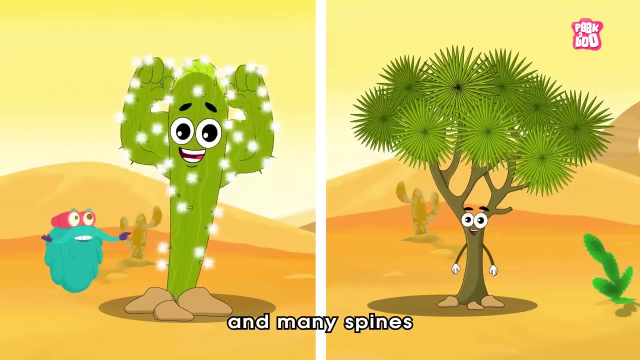 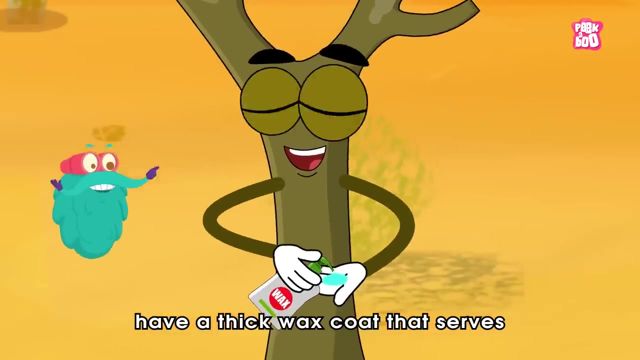 starting with plant adaptation in deserts. As we know, the desert has scarcity of water with dry land. thus, the plants like the thorny cactus and Joshua tree have small or no leaves and many spines that help them conserve water. These tiny leaves have a thick wax coat that serves to retain water for a long time, while 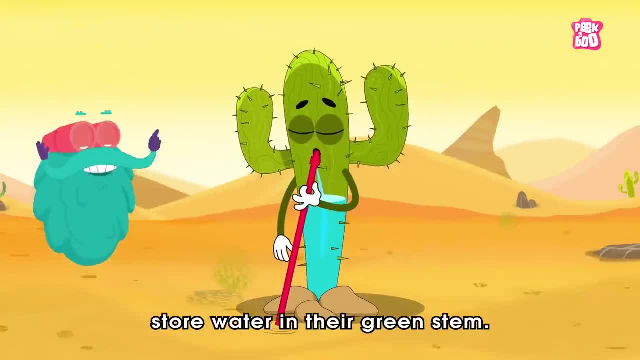 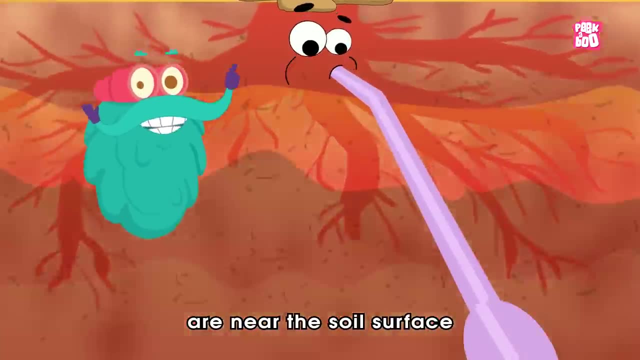 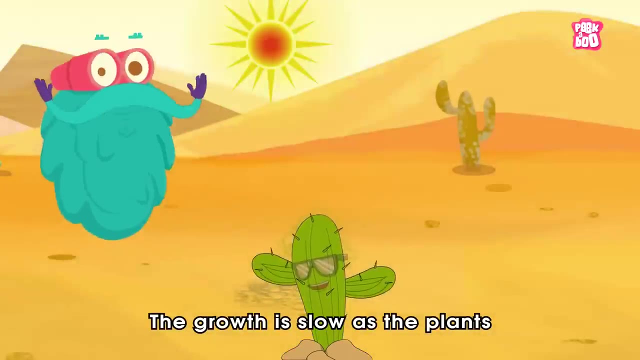 the leafless plants, like cactus, store water in their green stem. Also, the roots of these desert plants are near the soil surface. that help to soak up water before it evaporates in the sky. The growth is slow as the plants do not have to make much food. 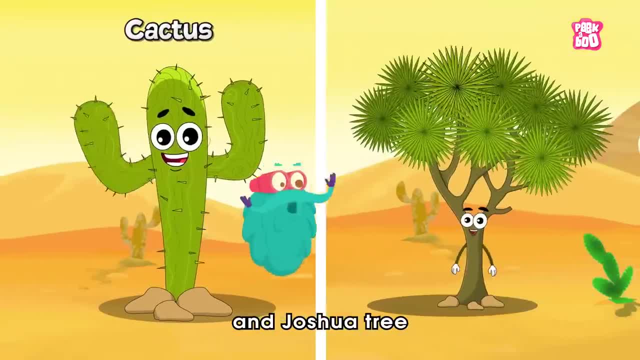 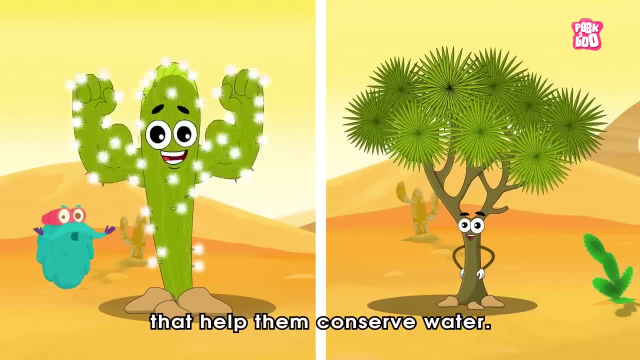 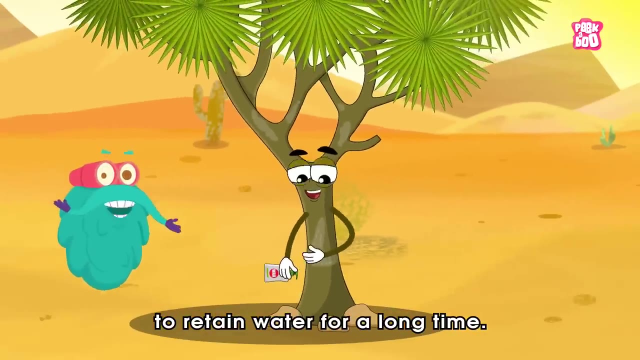 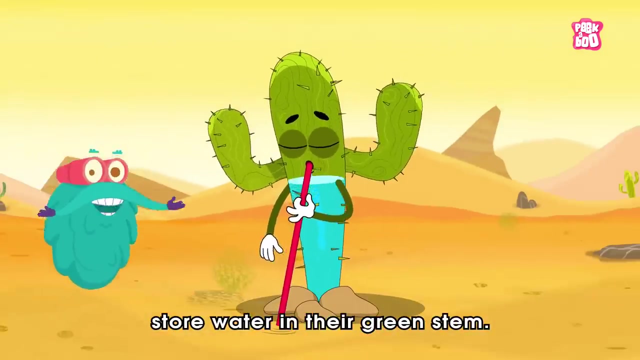 Thus, the plants like the thorny cactus and Joshua tree have small or no leaves and many spines that help them conserve water. These tiny leaves have a thick wax coat that serves to retain water for a long time, while the leafless plants like cactus store water in their green stem. 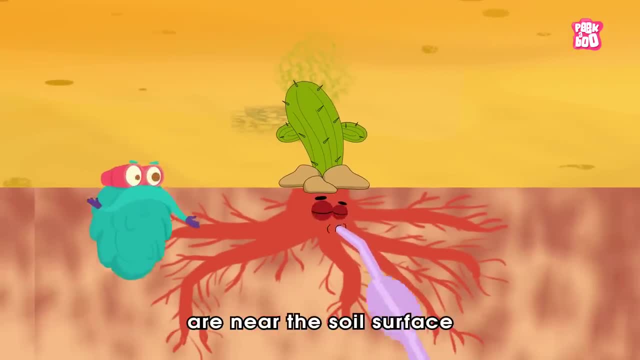 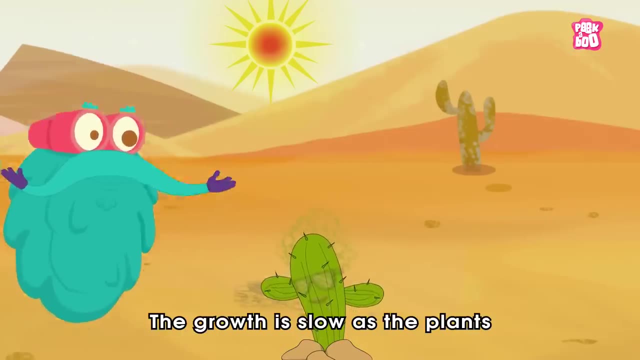 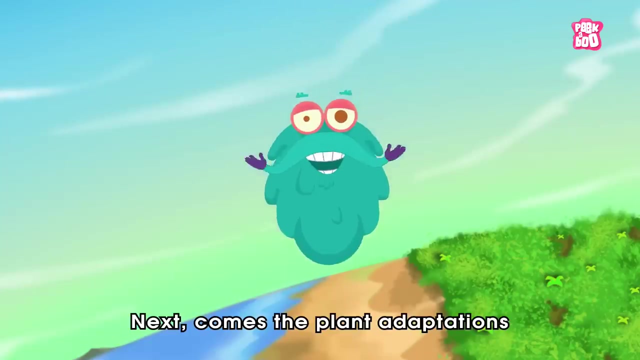 Also, the roots of these desert plants are near the soil surface that help to soak up water before it evaporates in the sky. The growth is slow as the plants do not have to make much food. Next comes the plant adaptations in the tropical rainforest. The tropical rainforest has a unique environment due to its hot climatic condition and heavy rain, which can cause problems such as promoting the growth of bacteria and fungi which could be harmful to plants. So the plants here have drip tips and waxy coverings on leaves to shed the extra water. 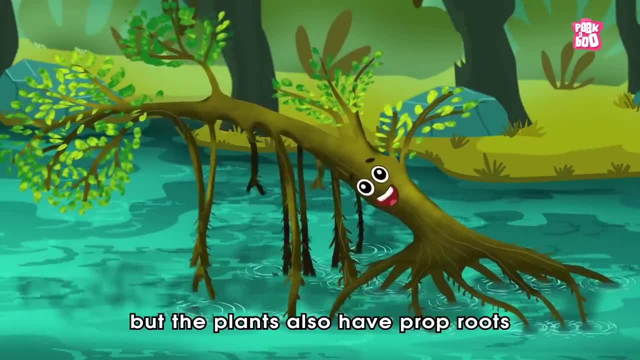 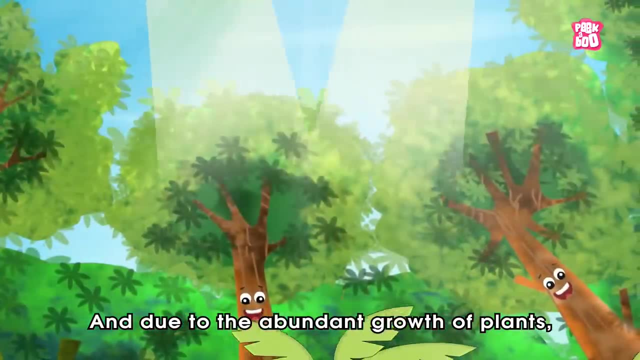 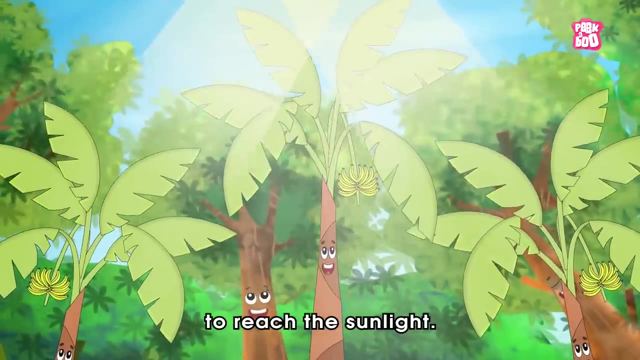 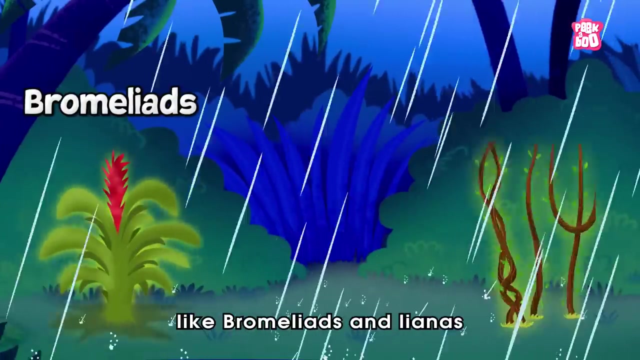 Not only that, but the plants also have prop roots that help support them in the shallow soil And, due to the abundant growth of plants, some plants grow on top of one another to reach the sunlight. The types of plants we can find in the tropical rainforest, like Bromeliads and Lianas, 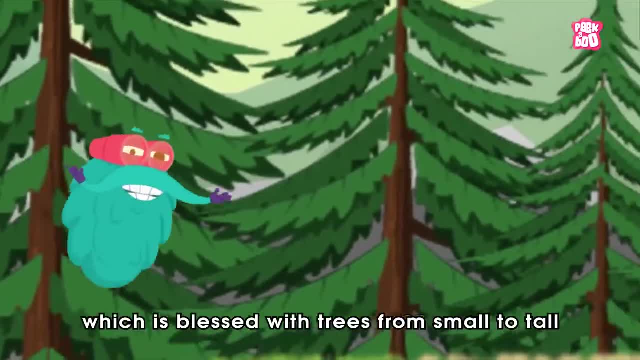 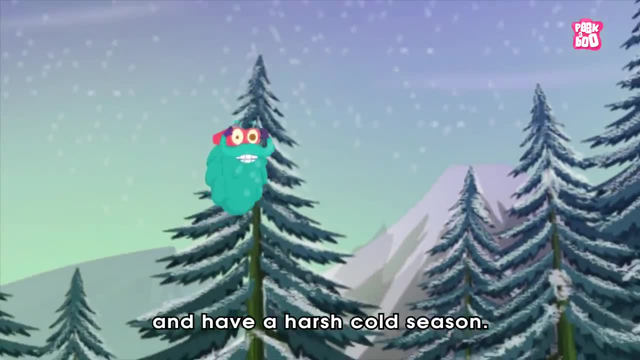 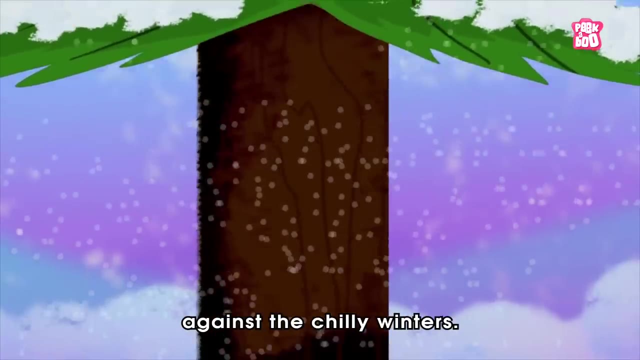 Let us move further towards the temperate forest. The temperate forest, which is blessed with trees from small to tall, that witnesses four distinct seasons and have a harsh cold season. So most big trees here have thick barks to shed them against the chilly winters. 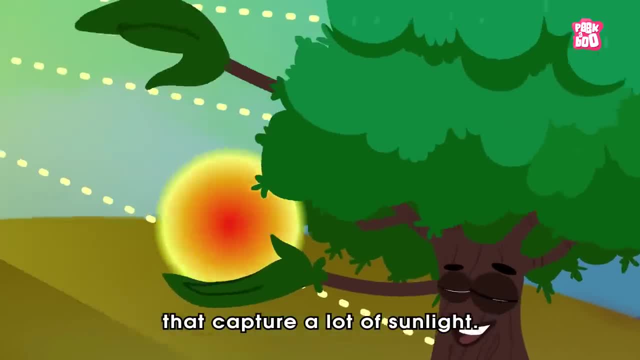 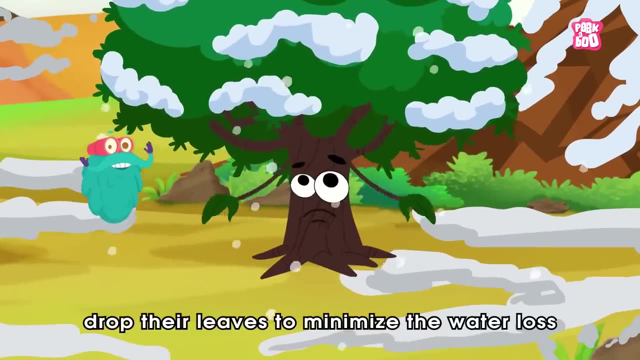 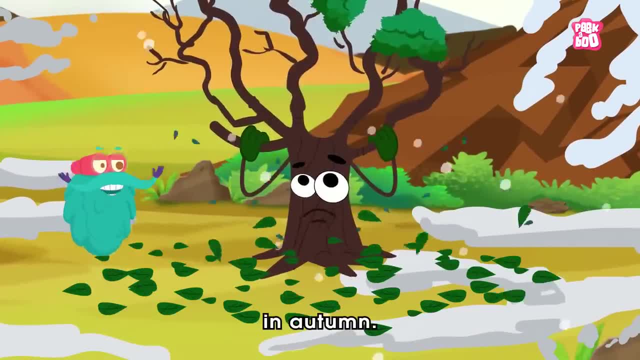 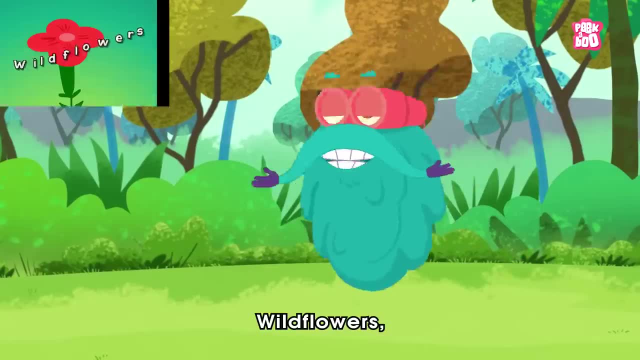 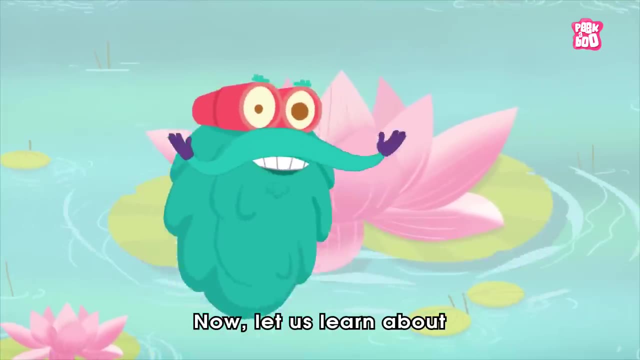 They also drop their leaves to minimize the water loss in autumn. Now that's really smart. Some examples of the kind of trees found here are wild flowers, oak ash, maple, etc. Now let us learn about plant adaptation in water. 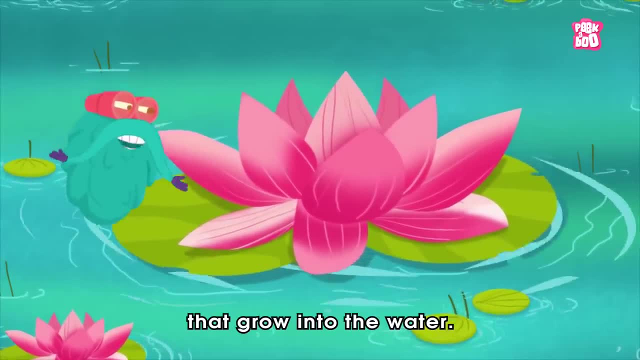 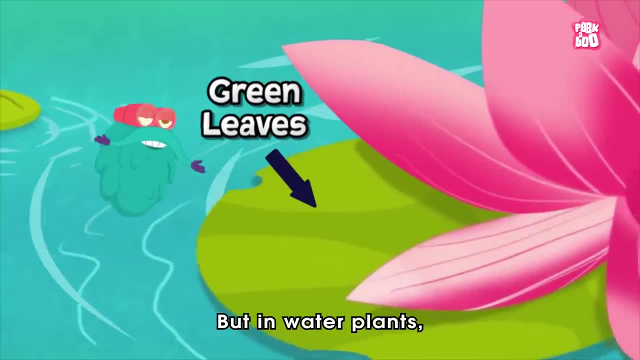 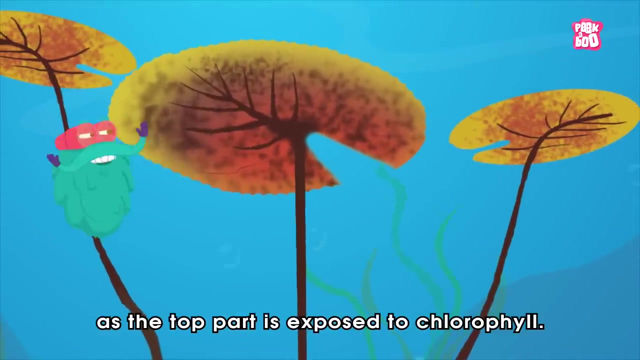 You see, things are a bit different. in plants that grow into the water, We all have seen- the leaves are green in color. But in water plants the leaves are greener on the upper side, whereas red in lower portions, as the top part is exposed to chlorophyll. 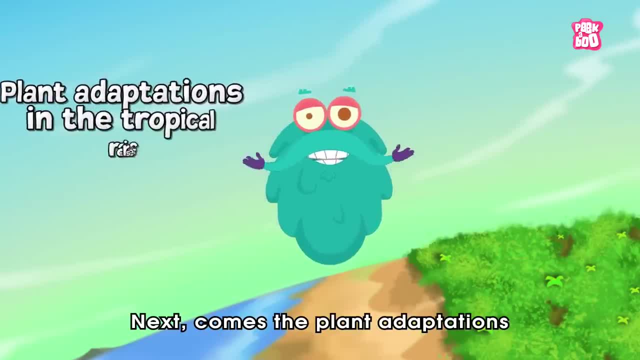 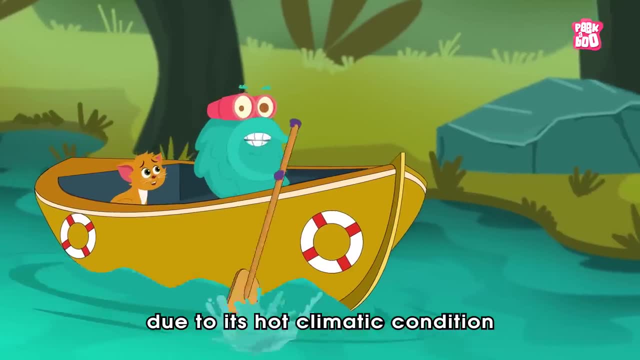 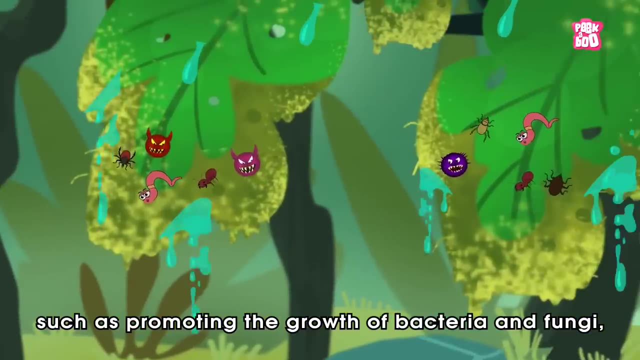 3. Plant Adaptation in the Tropical Rainforest. The tropical rainforest has a unique environment due to its hot climatic condition and heavy rain, which can cause problems such as promoting the growth of bacteria and fungi, which could be harmful to plants. 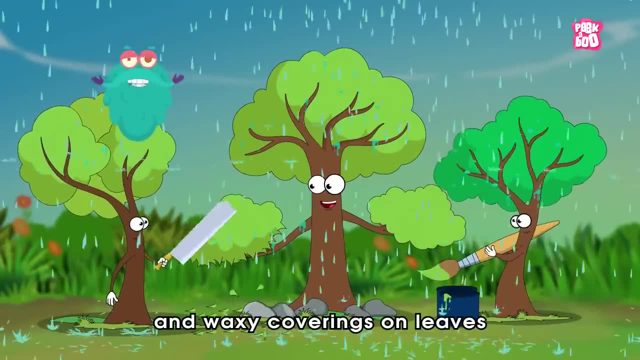 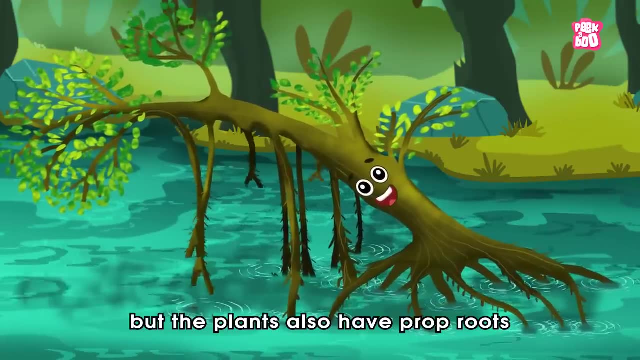 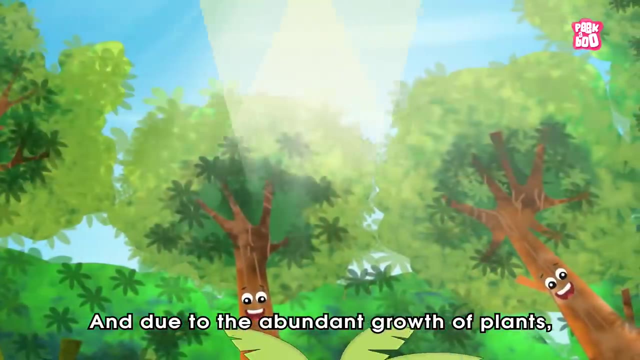 So the plants here have drip tips and waxy coverings on leaves to shed the extra water. Not only that, but the plants also have prop roots that help support them in the shallow soil. And due to the abundant growth of plants, some plants grow on top of one another to 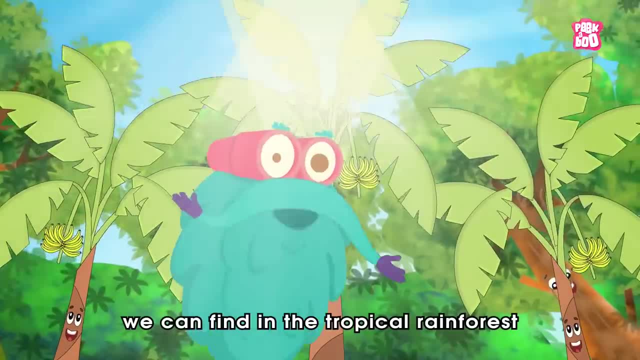 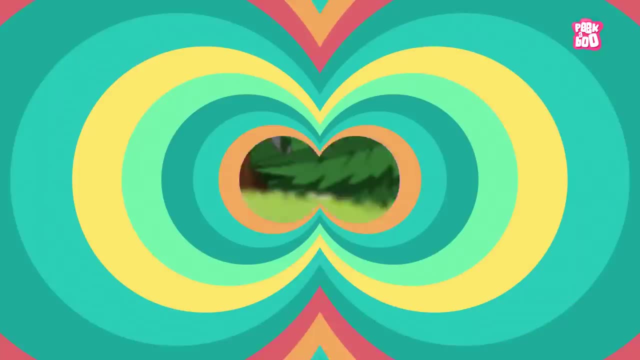 reach the sunlight, The types of plants we can find in the tropical rainforest, like Bromeliads and Lianas. Let us move further towards the temperate forest. This forest is known as the tropical rainforest, which is blessed with trees from small to. 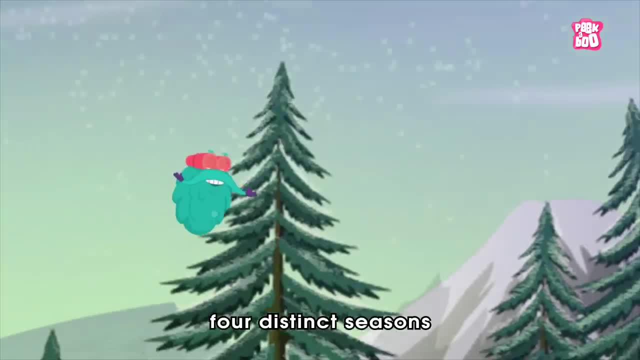 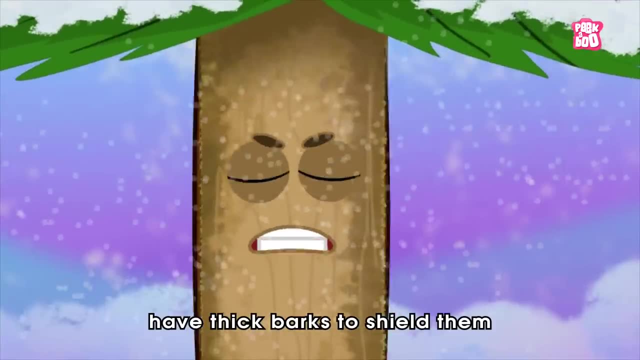 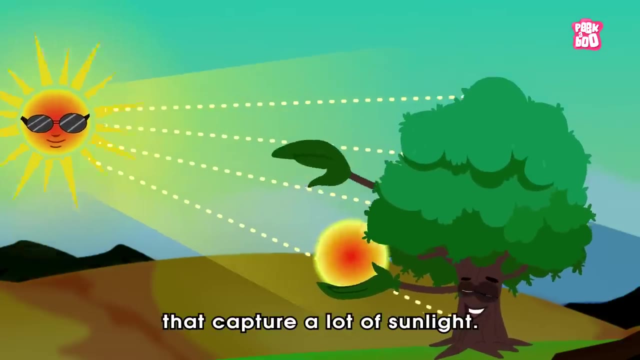 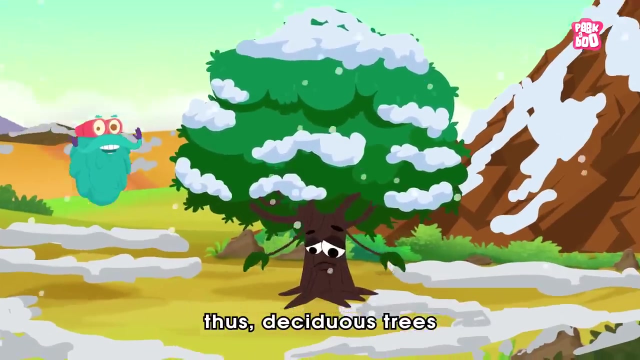 tall that witness four distinct seasons and have a harsh cold season. So most big trees here have thick barks to shed them against the chilly winters. Also, they have broad leaves that capture a lot of sunlight, But these leaves can weigh down the trees in winter. thus deciduous trees drop their 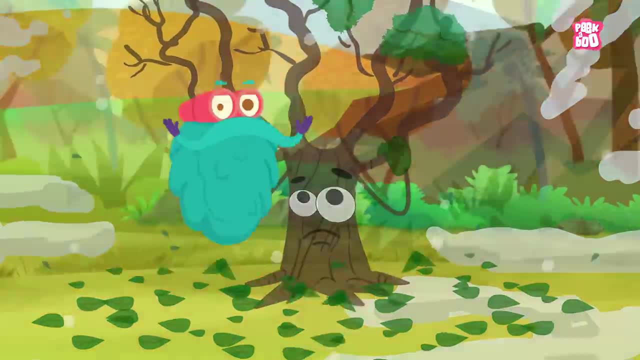 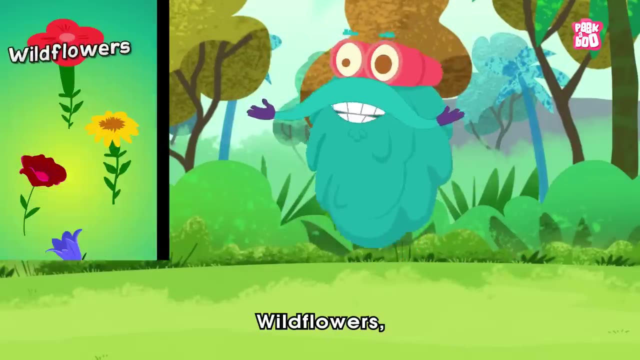 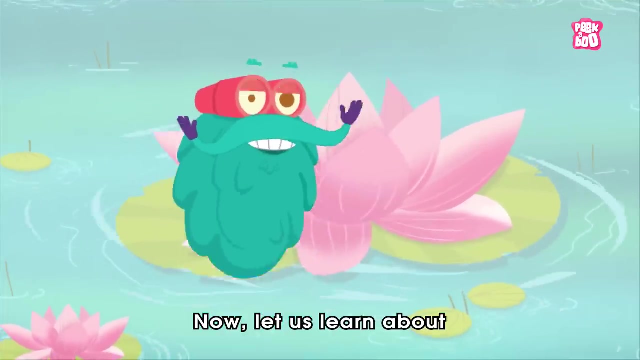 leaves to meet the sun. This is to minimize the water loss in autumn. Now, that's really smart. Some examples of the kind of trees found here are wildflowers, oak, ash, maple, etc. Now let us learn about plant adaptation in water. 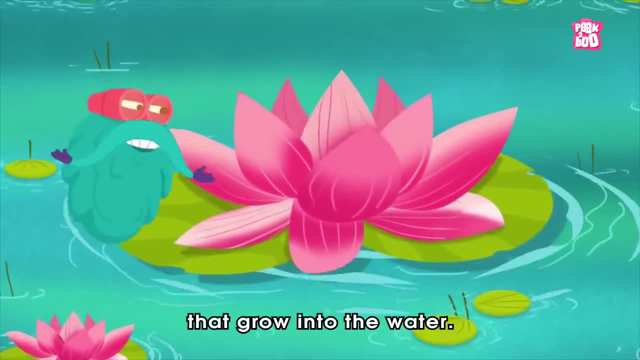 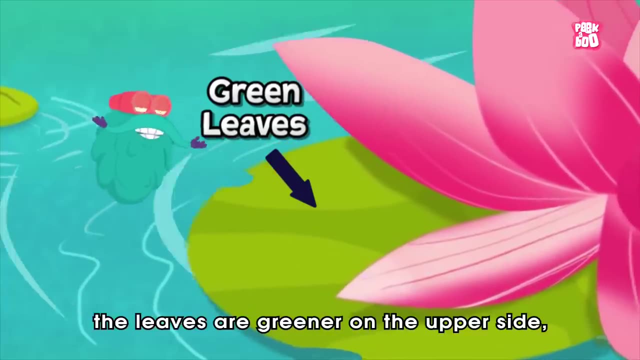 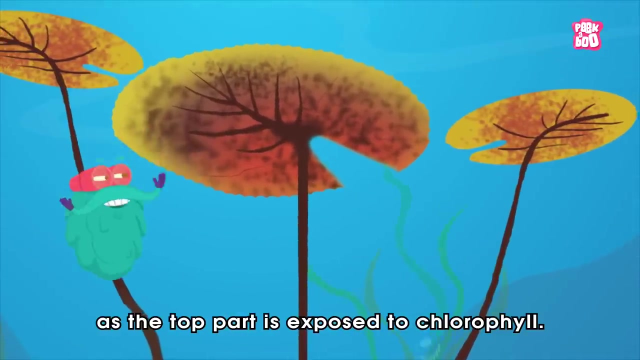 You see, things are a bit different. in plants that grow into the water, We all have seen- the leaves are green in color. But in water plants the leaves are greener on the upper side, whereas red in lower portions, as the top part is exposed to chlorophyll. 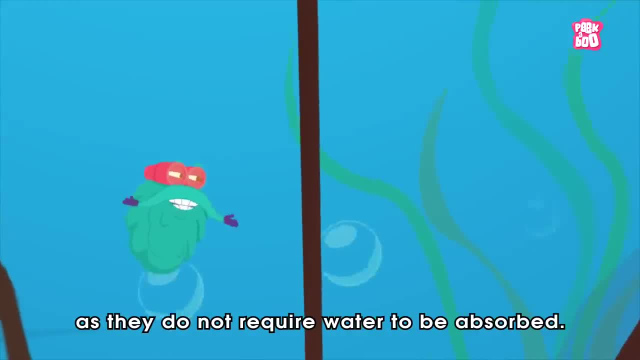 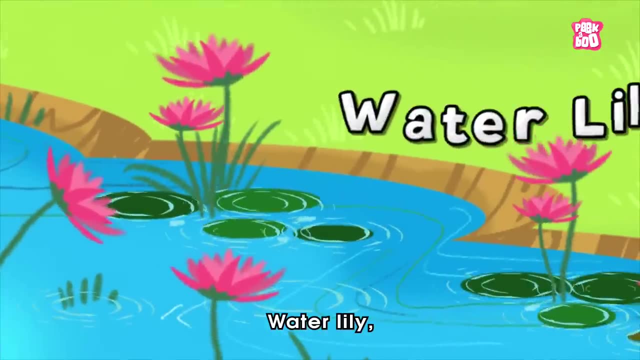 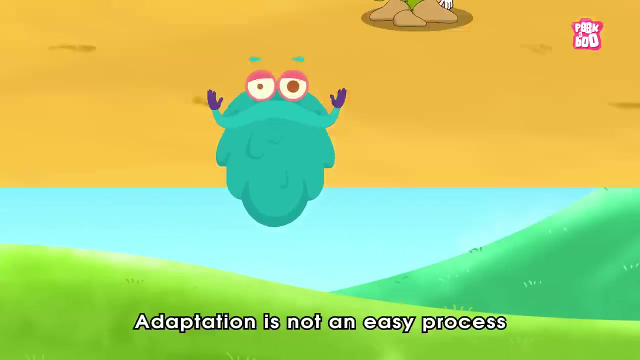 Also, these plants do not have stems, as they do not require water to be absorbed. Some examples of these beautiful plants are water lily and lotus. So, in conclusion, Adaptation. Adaptation is not an easy process and takes time to develop.